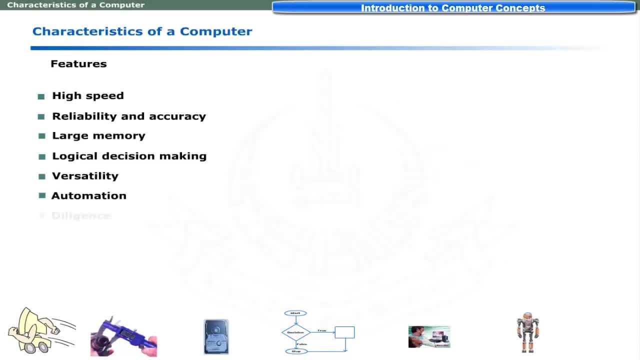 versatility, automation and diligence. First feature of computer is its speed. The speed of personal computer is measured in terms of megahertz, That is millions of clock cycles generated by microprocessor clock in one second. Most modern microcomputers are rated from: 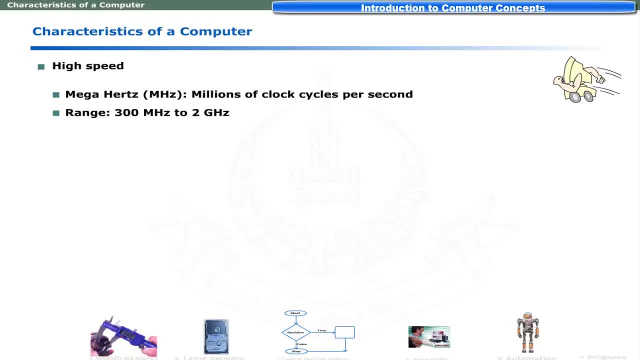 300 to 100.. A typical 800 megahertz computer takes a very small fraction of a second to complete one cycle. Normally, several clock cycles are required to fetch a single instruction from memory, decode it and execute it. The speed of workstations, mainframes and high-speed 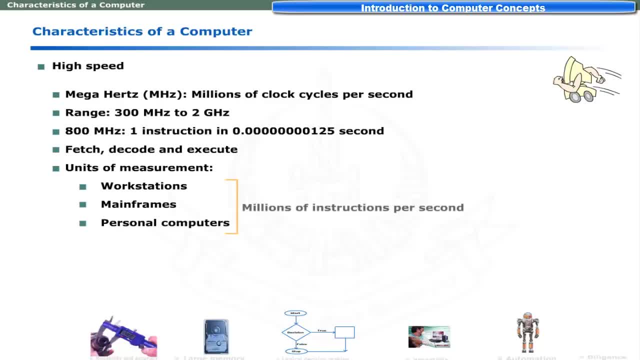 personal computers is measured in terms of millions of instructions per second. These computers operate in the range of 20 to 1000 MIPS. Typically, a 100 MIPS computer can execute 100 million instructions per second. The speed of supercomputer is measured in terms of floating point operations per second. 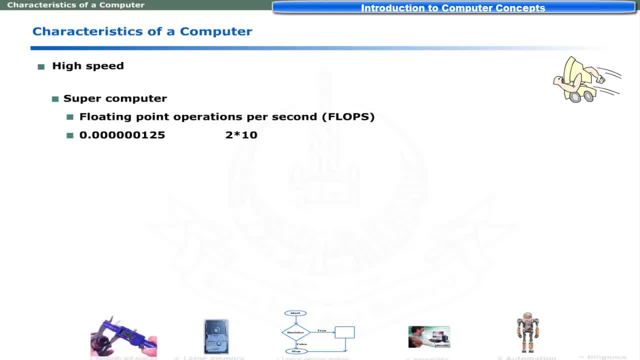 Floating point numbers include very small or very large numbers. Super computers operate at a speed of 500 gigaflop to 3 teraflops. A gigaflop is 1 billion flops and a teraflops is 2 gigaflop. Now we will discuss some characteristics of computers. blows signal speed with J V, J cup, EM, Tc, Tm, R, K, V, Q, V that we use every single second within our computing cycle. Most computers tender at chamber value Thence时 nei ten Greene I I, Ursula K I. 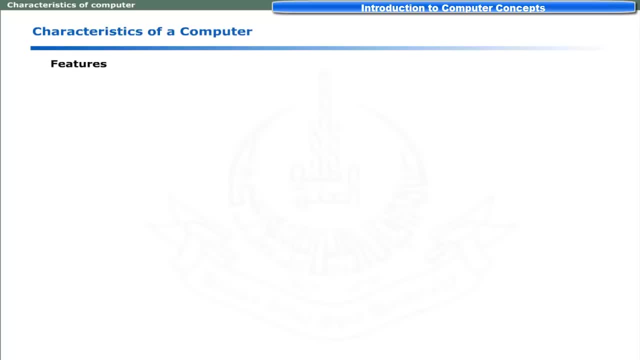 Some features of computers are high speed, reliability, accuracy, large memory, logical decision-making, versatility, automation and diligence. First feature of computer is its speed. The speed of personal computer is measured in terms of megahertz, That is, millions of clock cycles generated by microprocessor clock in one second. 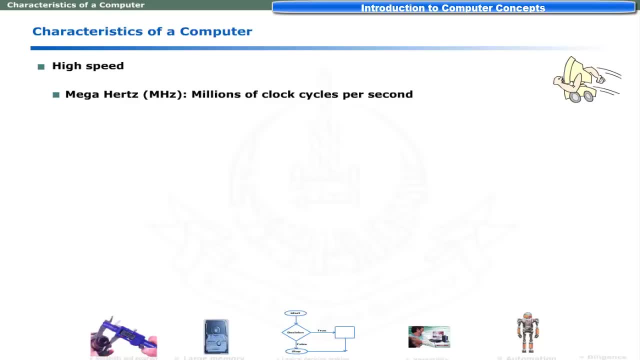 Most modern microcomputers are rated from 300 megahertz to 2 gigahertz. A typical 800 megahertz computer takes a very small fraction of a second To complete one cycle. normally, several clock cycles are required to fetch a single instruction from memory, decode it and execute it. 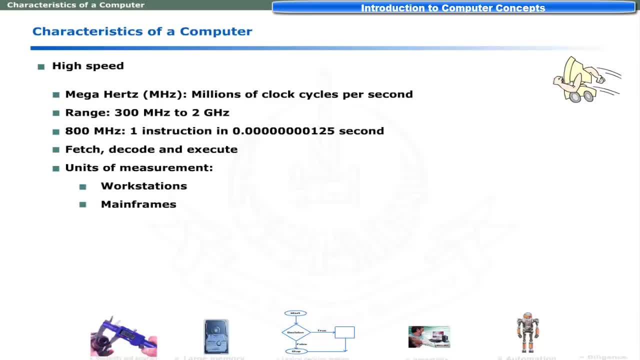 The speed of workstations, mainframes and high speed personal computers is measured in terms of millions of instructions per second. These computers operate in the range of 20 to 1000 gigahertz. Typically, a 100-mips computer can execute 100 million instructions per second. 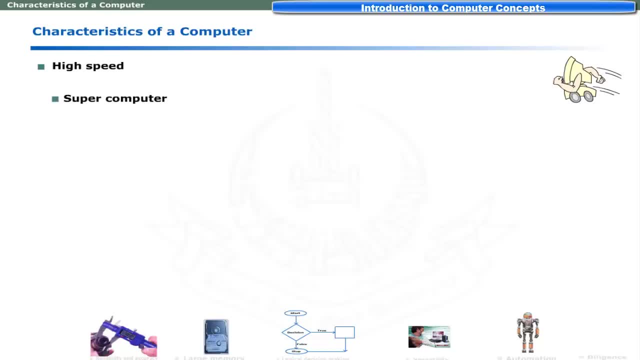 The speed of supercomputer is measured in terms of floating-point operations per second. Floating-point numbers include very small or very large numbers. Supercomputers operate at a speed of 500 gigaflops to 3 gigaflops. A gigaflop is 1 billion flops and a teraflop is equal to 1 trillion flops. 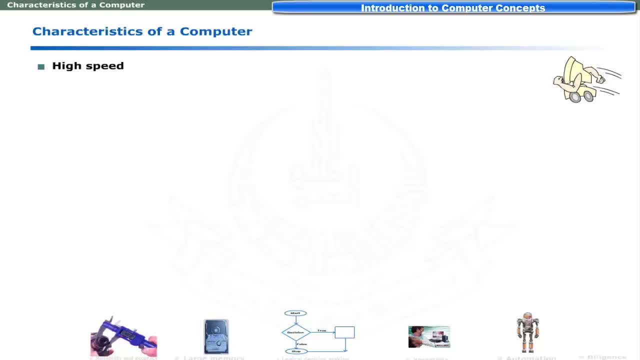 Second and the most important feature of computer is reliability and accuracy. The results of computers are highly reliable and precise. Computers maintain accuracy within a millisecond, microsecond and second. It is also very important to be able to calculate the exact number of seconds, nanosecond, picosecond or any level of required precision. 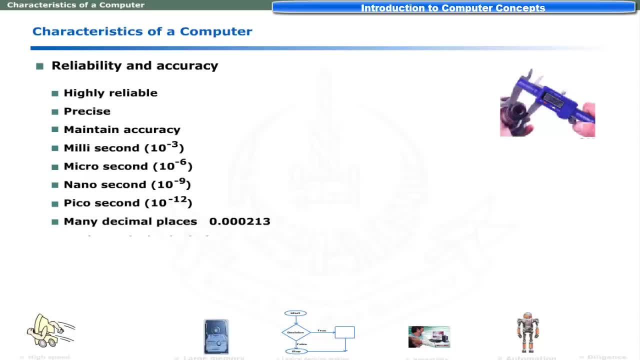 These are also accurate up to many decimal places in mathematical calculations. High accuracy and reliability is because a computer works on electrical pulses that rarely fail to convey correct information. The reliability of computers is maintained. The reliability of computers is maintained, especially in repetitive tasks. 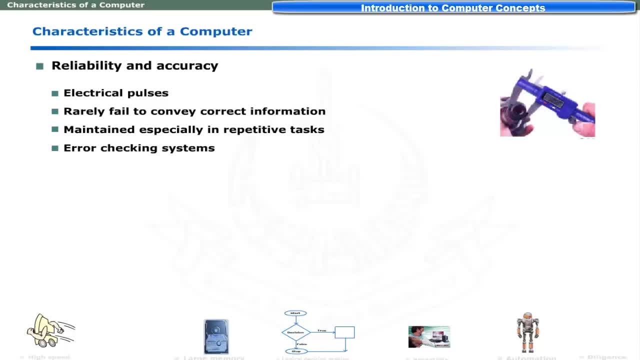 Further, the error-checking systems are built in the computer to reduce the chance of errors. Organizations provide backup computers that automatically take over in case the main computer fails. Recovery systems are implemented to further strengthen the reliability of data. Dear learners, another feature of computer is its large memory. 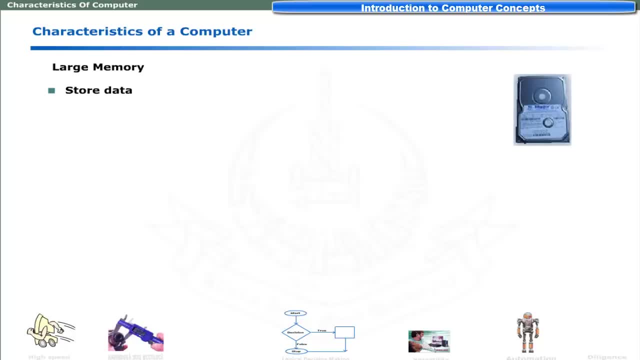 Computer memory is used to store data and information temporarily or permanently. Temporary memory is normally referred to as random access memory. This is used to temporarily store programs that are currently executed. The contents of RAM are erased when the power is off. Normally, the size of temporary memory is measured. 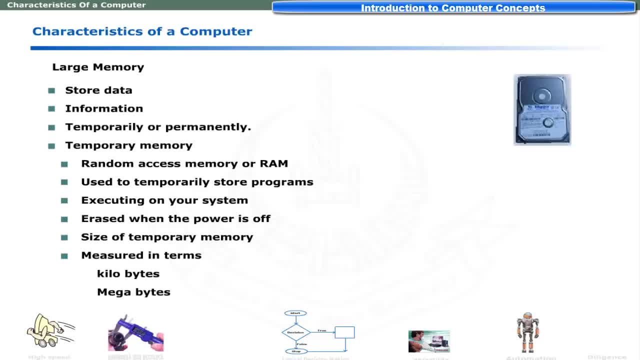 in terms of kilobytes and megabytes. Most modern computers and special graphics computers have large memories in multiples of gigabytes. Permanent memory is used to permanently store data and store large repositories of data, user programs, applications like MS Office and operating systems. 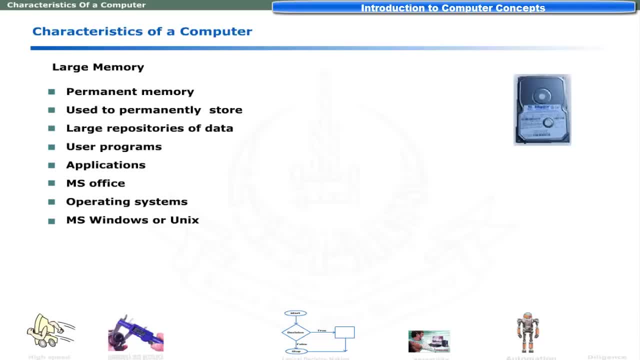 like MS Windows or Unix. An example of permanent storage is hard disk. The programs stored on permanent memory are available when you switch on the computer. Large amount of data can be stored on permanent storage devices. Computer memories have another advanced feature: to dynamically access any data, irrespective of its storage location. 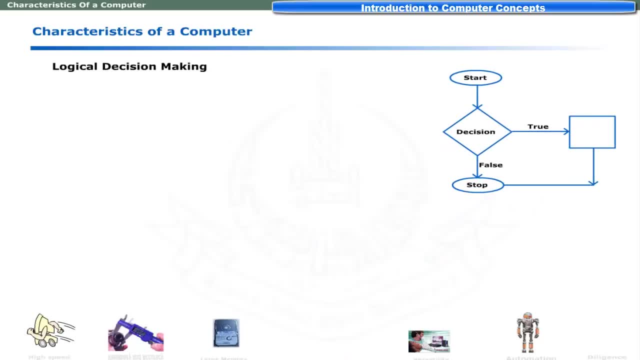 Apart from computations, a computer has the ability to take decisions. The computer has special circuits to perform logical operations. Logical operations include comparisons such as: a number is equal to, greater than or less than another number, Depending upon the results of logical operations. 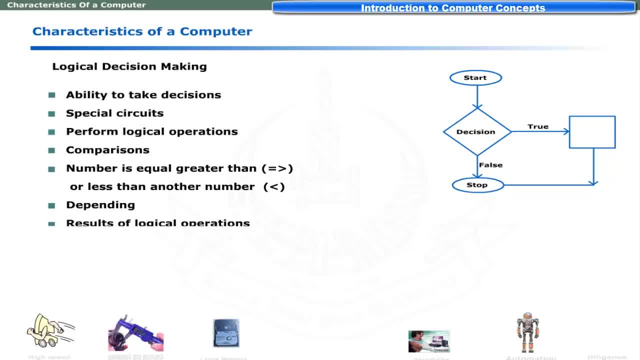 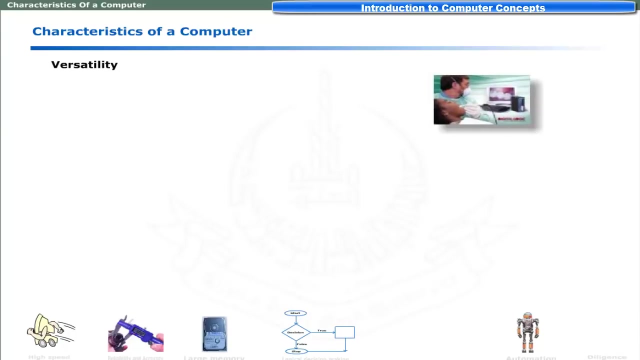 a computer can take appropriate actions. Computer is also capable of comparing text, images and even audio. The decision-making capabilities of computer has led to the invention of artificial intelligent machines. Computer is a versatile machine. It is capable of solving a variety of problems. 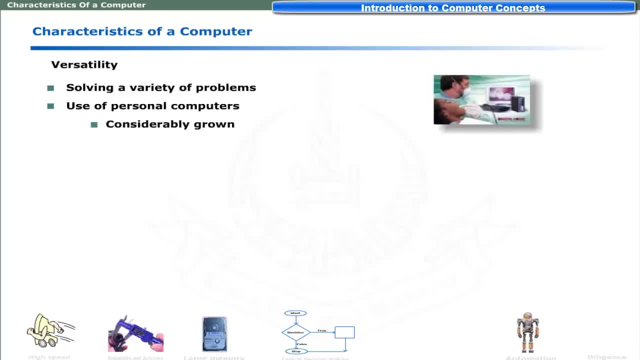 The use of personal computers have considerably grown in the fields of communications, multimedia, scientific research, designing, engineering, education and entertainment. Another remarkable feature of computers is its ability to perform operations automatically. When the computer is switched on, it automatically executes instructions to check all peripheral devices. 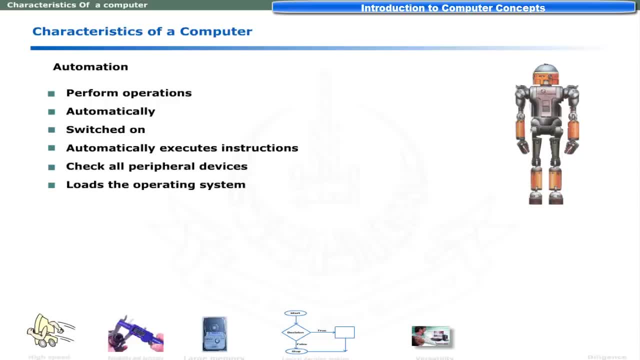 loads the operating system and provides interface to the user without human interaction. Computer is a diligent machine. It never feels tiredness. You can complete different jobs or a single task repeatedly without losing perspective. Some computer systems are rarely down in several years. 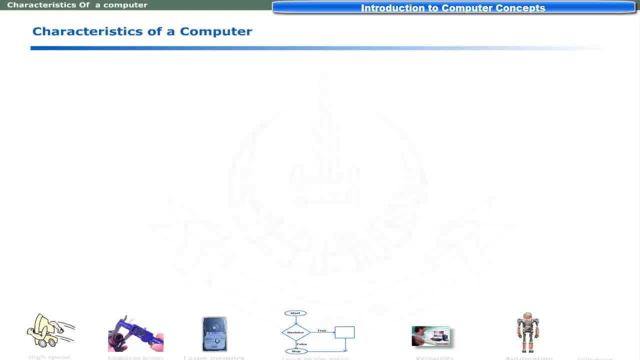 These can process data continuously and accurately. Dear learners, Although computers are widely used due to their versatility, but computers have certain limitations. Some limitations of computers are lack of intelligence, need of proper environment for smooth operation and need of special language. The first limitation of computer is its lack of intelligence. 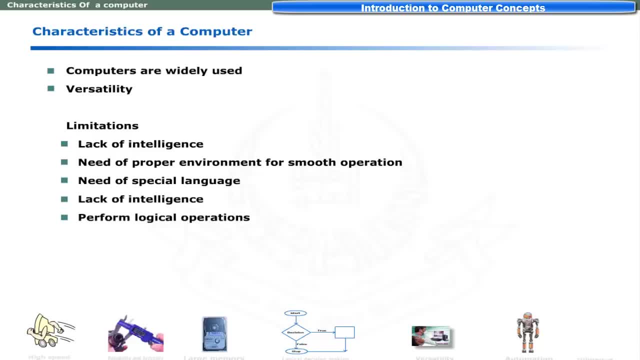 Although a computer can perform logical operations at a very fast speed, but it is unable to think like a human. Presently, computers cannot tell the fragrance of a flower or have no aesthetic sense. Computers need proper environment for smooth operations. These can only operate in dust-free environment. 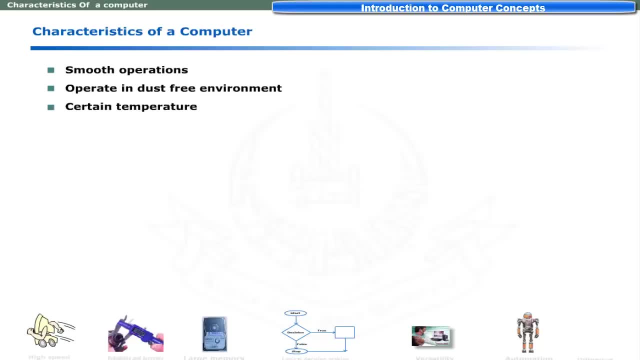 under certain temperature conditions. Computers can only understand binary codes, that is, zeros ones and their combinations. These codes are not commonly used by humans. Special software, interpreters and compilers are used to convert natural languages to computer-understandable codes. Despite these limitations, 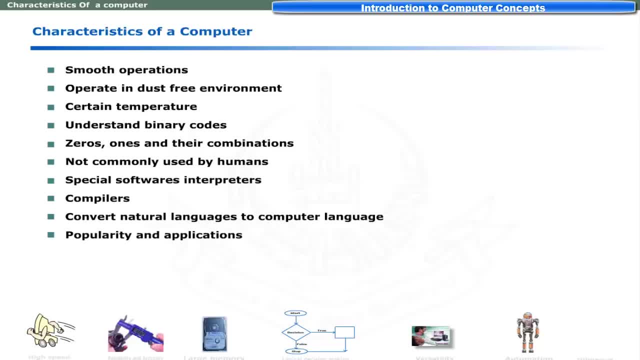 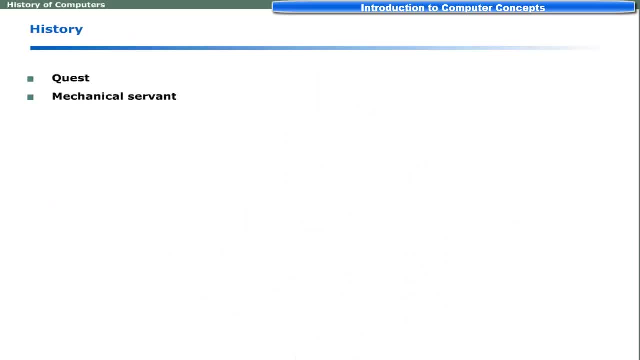 the popularity and applications of computers are considerably growing. Dear learners, The quest for a mechanical servant that could free people from tedious aspects of thinking is centuries old. It started with the introduction of abacus some 5,000 years ago. Abacus is considered the original manual counting device. 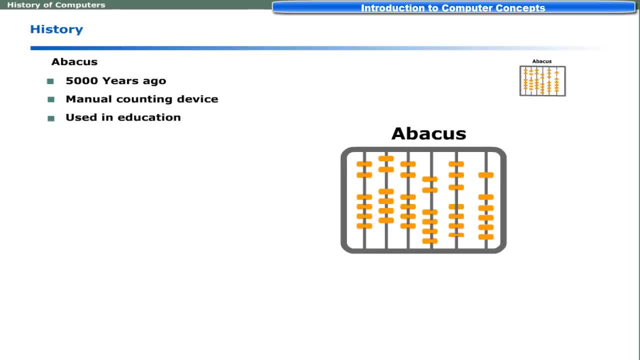 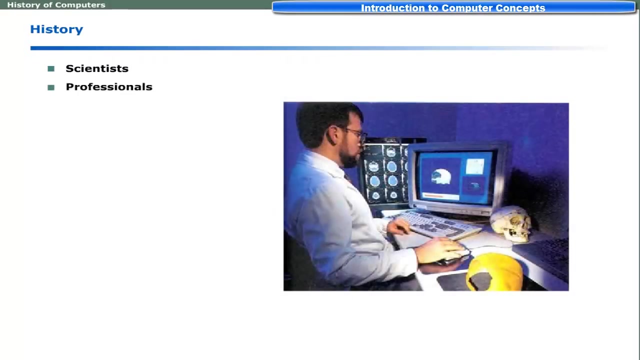 It is still used in education to demonstrate the principles of arithmetic. This device contains beads on rods. Calculations are made by positioning the beads upward or downward. Dear learners, Now we will discuss the contributions of scientists, professionals and students who contributed to bring to us this marvel of the modern age. 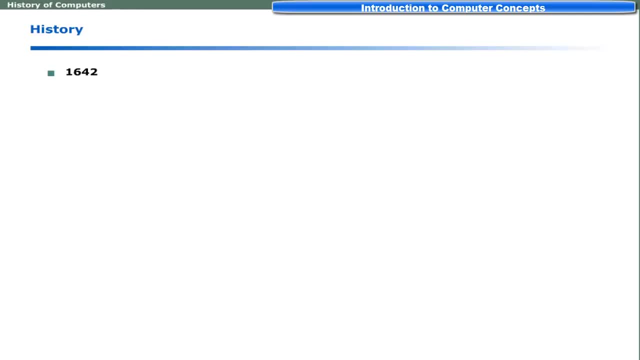 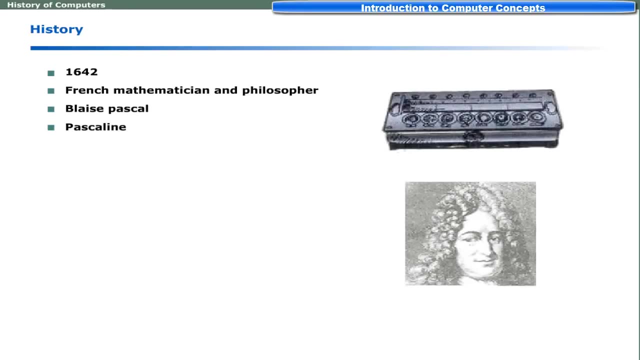 In 1642, French mathematician and philosopher Blaise Pascal invented Pascaline. It used wheels like telephone dials. Numbers were arranged on these dials. Wheels were evolved to make calculations. In 1801, a French weaver named Joseph-Marie Jacquard created Jacquard loom. 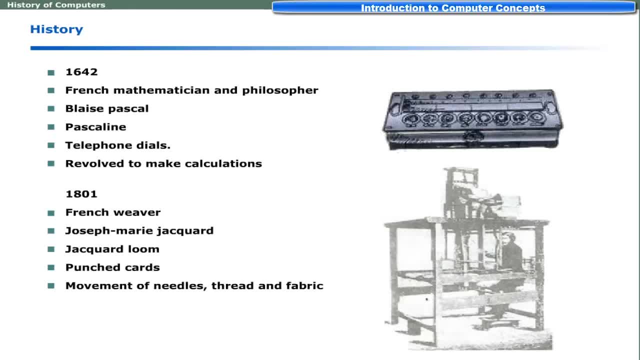 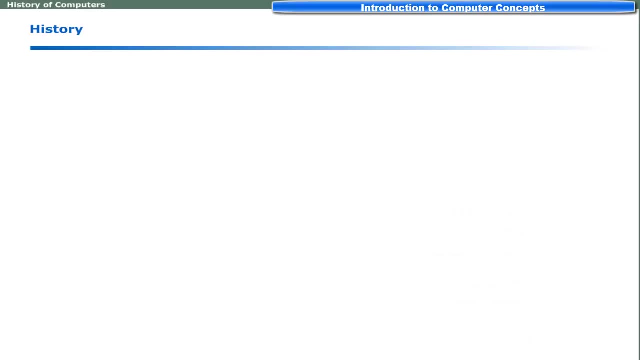 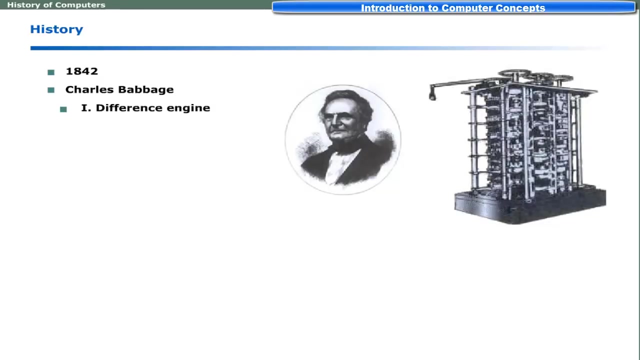 Punched cards were used to direct the movement of needles, thread and fabric. to create different patterns in a fabric on a loom known as Jacquard weaves. Efforts were made by different scientists across the world And in 1842, Charles Babbage introduced difference engine and then an analytical engine. 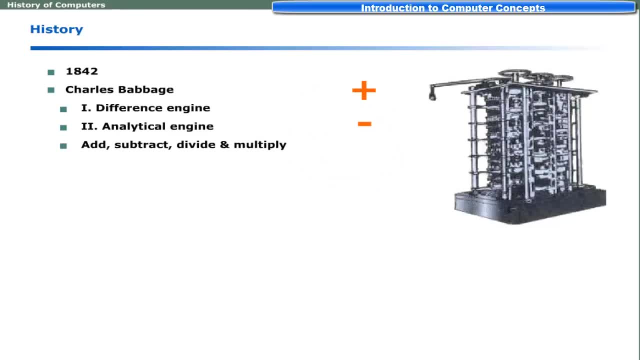 It was a general purpose computer that could add, subtract, divide and multiply in automatic sequence. Its average speed was 60 additions per second. The idea of Babbage was further refined and improved by Lady Ada Augusta Lovelace. She proposed that punched cards could be used to instruct Babbage's engine to perform repetitive tasks. 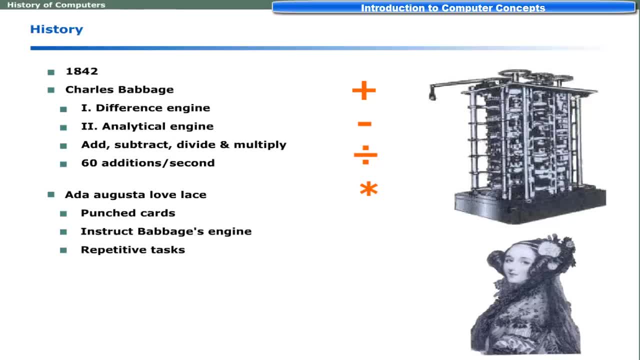 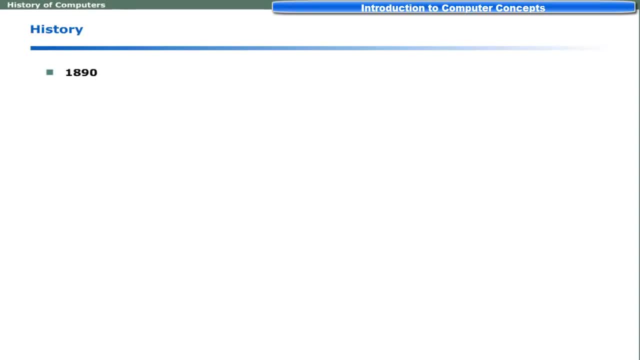 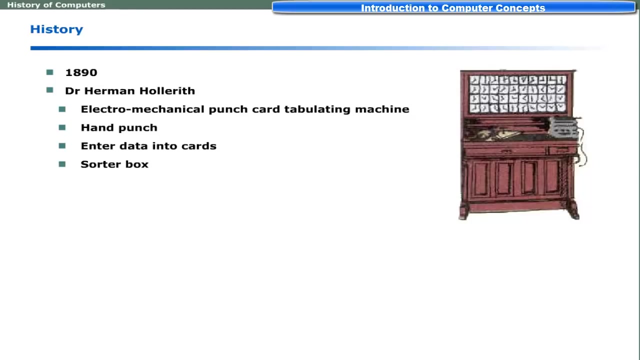 Due to her valuable contributions, she is considered as the first programmer. During 1890,, Dr Herman Hollerith developed the first electromechanical punch card technology. Handpunch was used to enter data into cards. A sorter box was used to read and sort these cards. 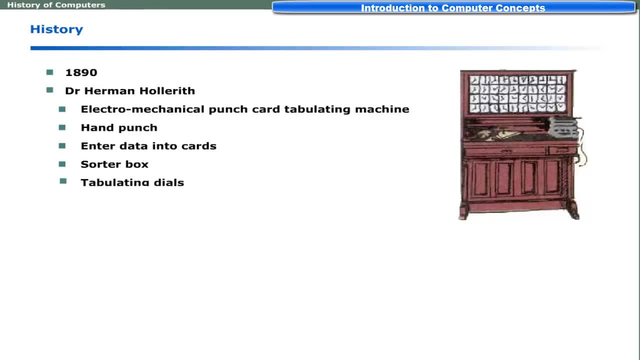 The output was summarized on tabulating dials. Hollerith earned handsome income by leasing his machinery to the governments of the USA, Canada, Austria and others. His invention led to the construction of a new machine. It led to the concept of modern data processing. 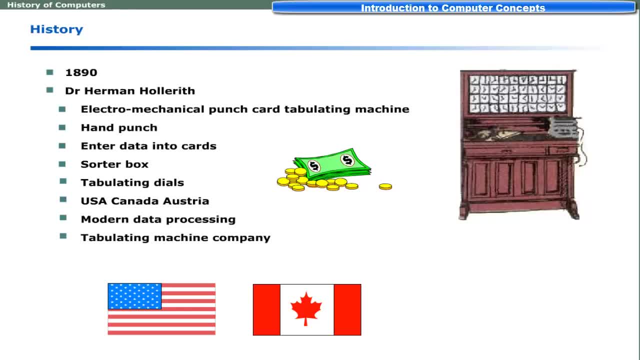 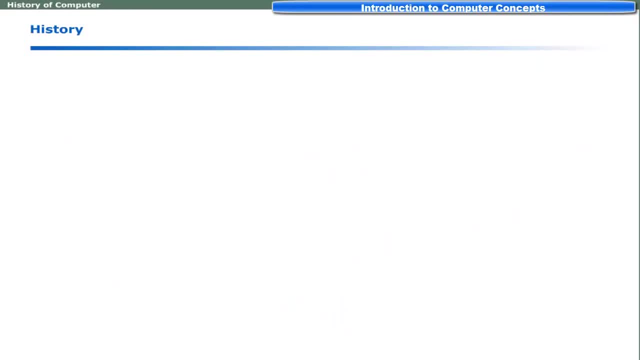 Hollerith is also the founder of tabulating machine company that later on became IBM Dear learners. sophisticated punch card devices were introduced from 1920 to 1950. The electromechanical accounting machine family included card punch verifier. reproducer. 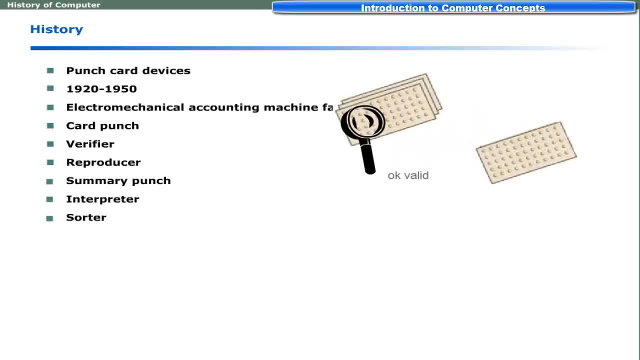 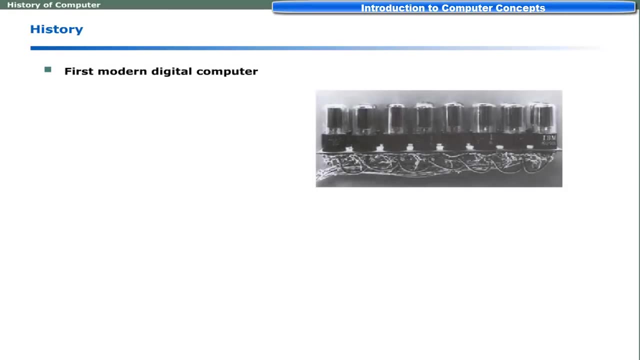 summary: punch interpreter, sorter, collater and accounting machines. These machines were very large, heavy and required physical labor to operate. The first modern digital computer, a Tanasov-Berry computer, was built in Iowa State University campus between 1939 and 1940.. 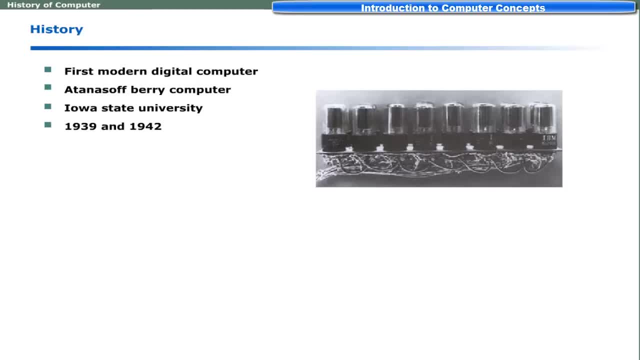 The development team was led by John Tanasov, professor of physics and mathematics, and a graduate student, Clifford Berry. This machine included many features like binary arithmetic, parallel processing, storage and computer functions. It weighed about 750 pounds and could store about 3,000 bits of data. 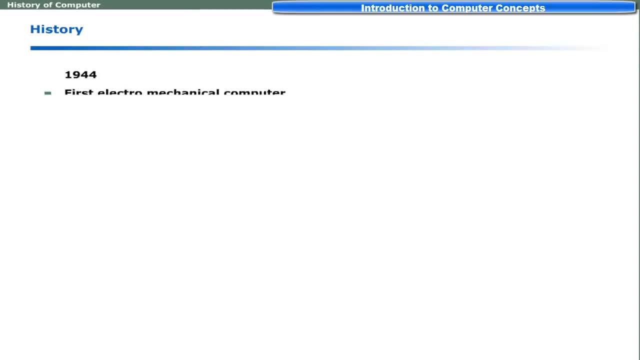 In the early 40s the first electromechanical computer, Mark I, was developed by Harvard University professor Howard Eichen. Dear learners, sophisticated punch card devices were introduced from 1920 to 1950. The electromechanical accounting machine family included. 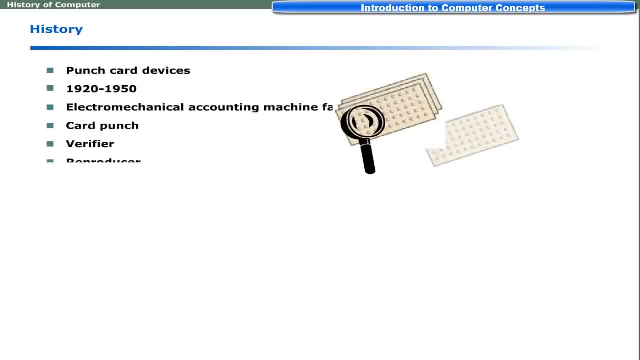 card punch verifier, reproducer, summary punch interpreter, sorter, collater and accounting machines. These machines were very large, heavy and required physical labor to operate. The first modern digital computer, a Tanasov-Berry computer, was built in Iowa State University campus between 1939 and 1942. 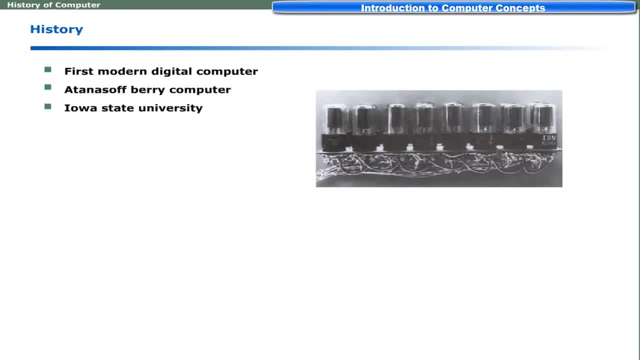 The first modern digital computer, a Tanasov-Berry computer, was built in Iowa State University campus between 1939 and 1942.. The first modern digital computer, a Tanasov-Berry computer, was built in Iowa State University campus between 1941 and 1942. 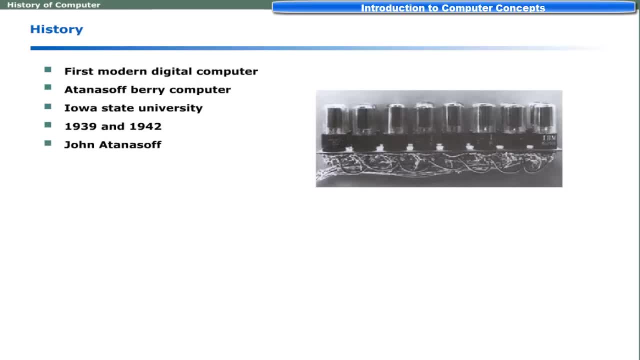 The development team was led by John Tanasov, professor of physics and mathematics, and a graduate student, Clifford Berry. This machine included many features like binary arithmetic, parallel processing, storage and computer functions. It weighed about 750 pounds and could store about 3,000 bits of data. 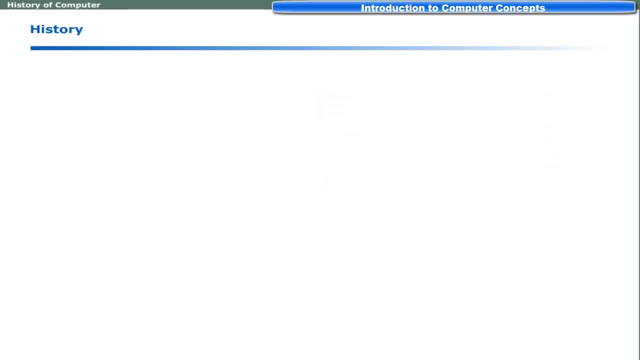 It weighed about 750 pounds and could store about 3,000 bits of data. In the early 40s, the first electromechanical computer, Mark I, was developed by Harvard University professor Howard Eichen. IBM sponsored the development of this huge machine. 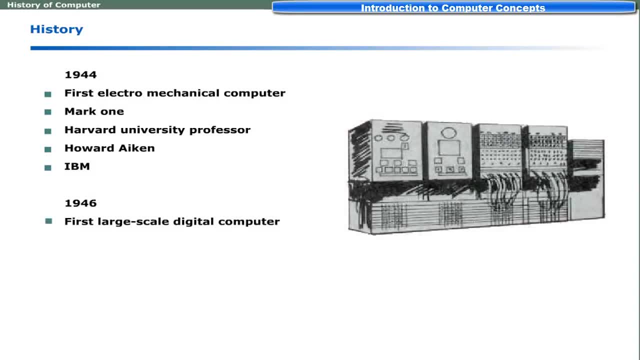 In 1946, first large-scale digital computer, the Electronic Numerical Integrator and Computer. In 1946, first large-scale digital computer, the Electronic Numerical Integrator and Computer. In 1946, first large-scale digital computer, the Electronic Numerical Integrator and Computer. 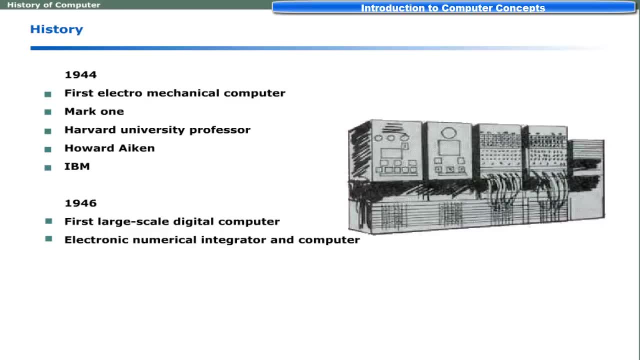 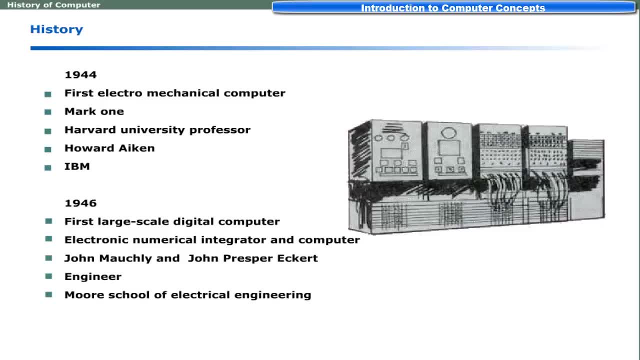 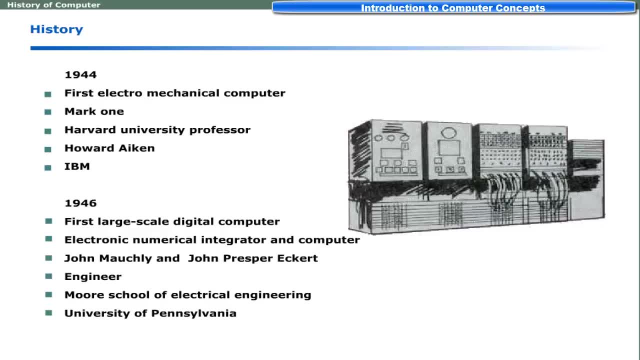 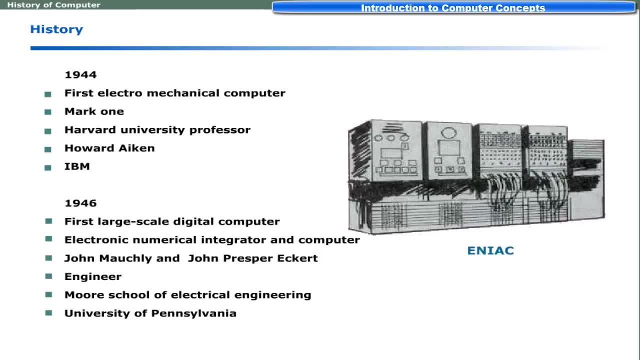 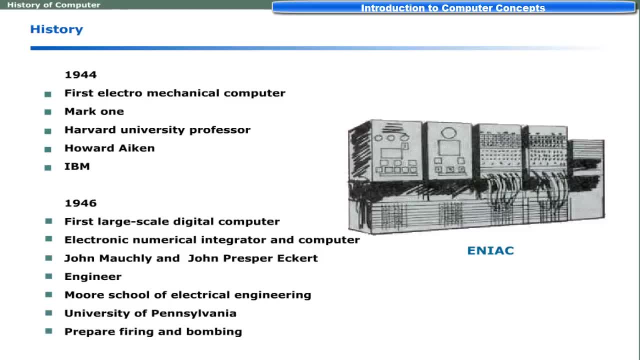 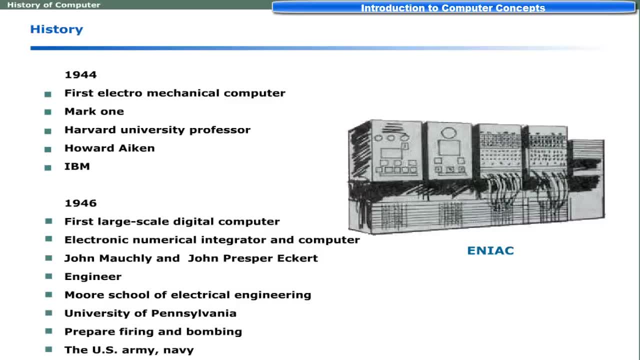 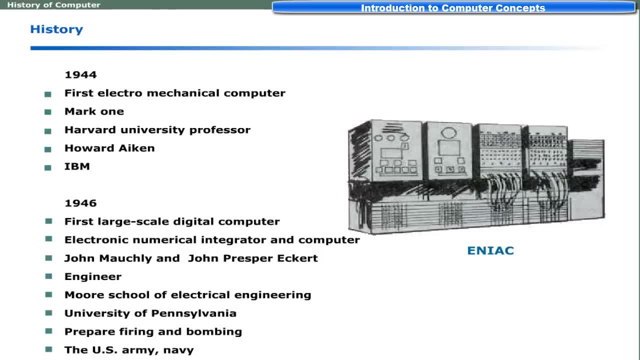 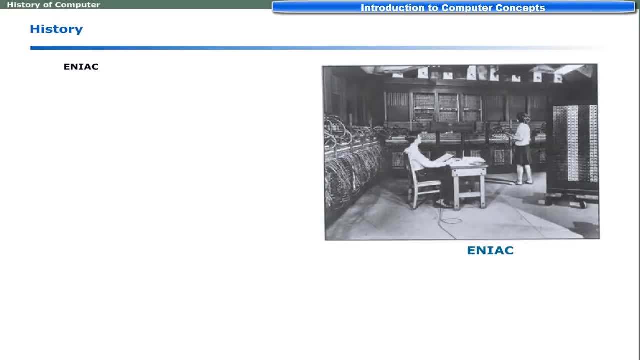 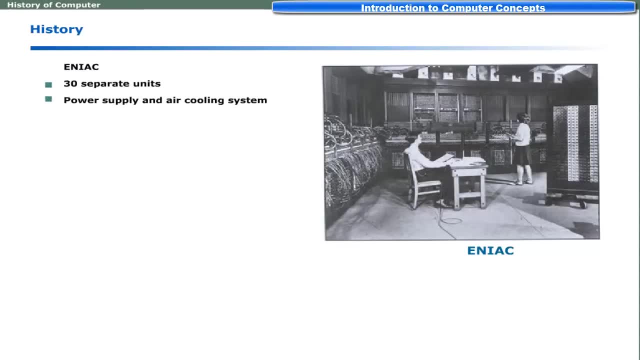 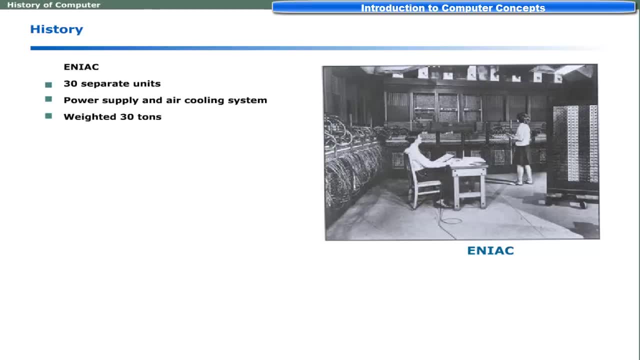 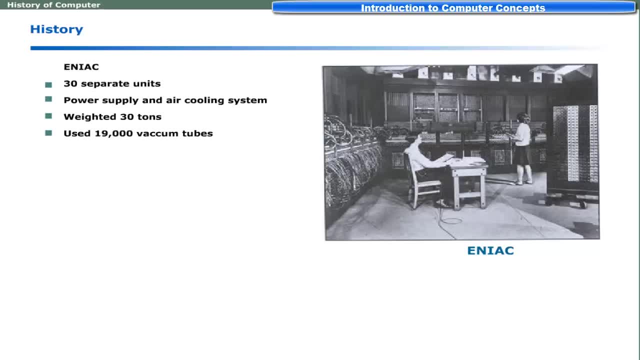 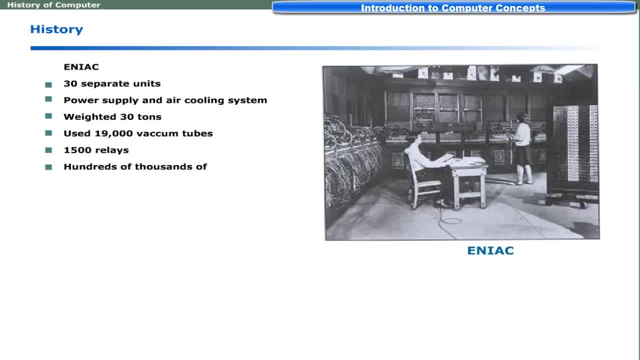 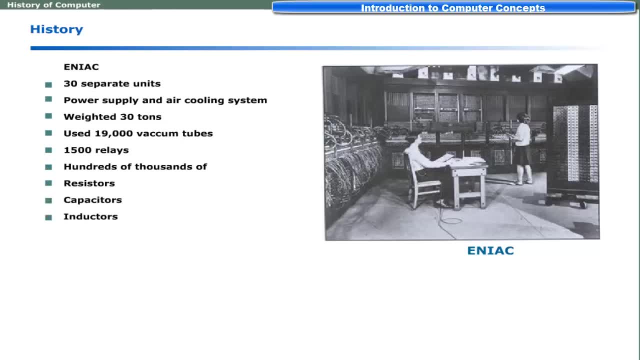 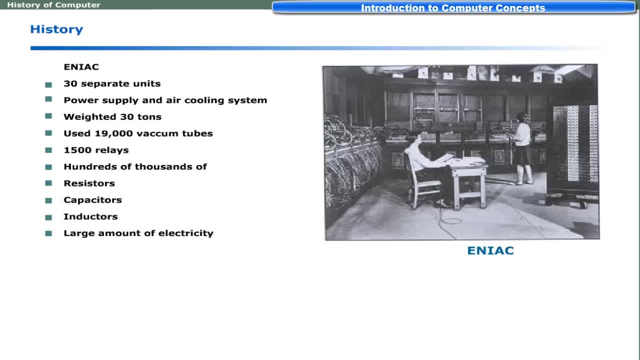 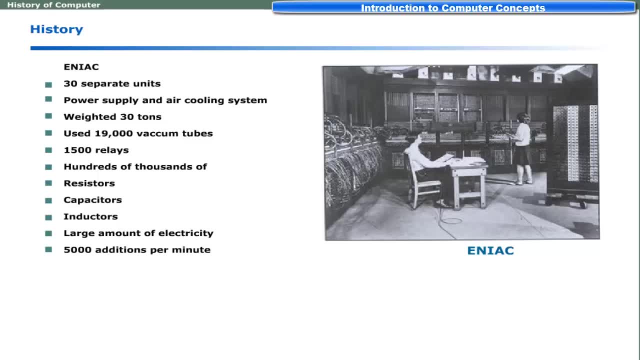 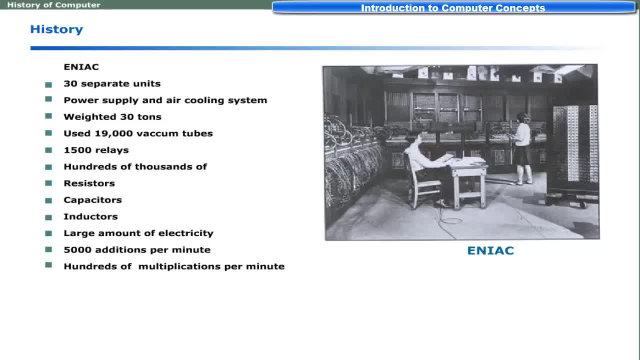 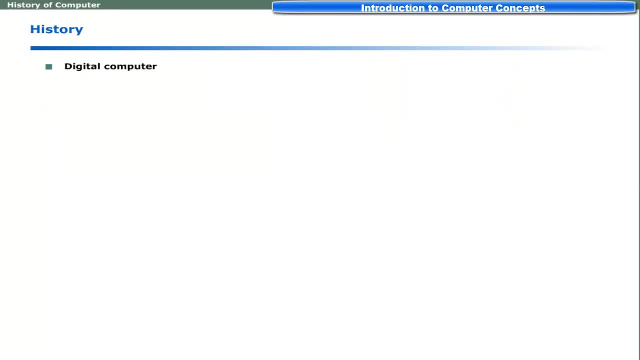 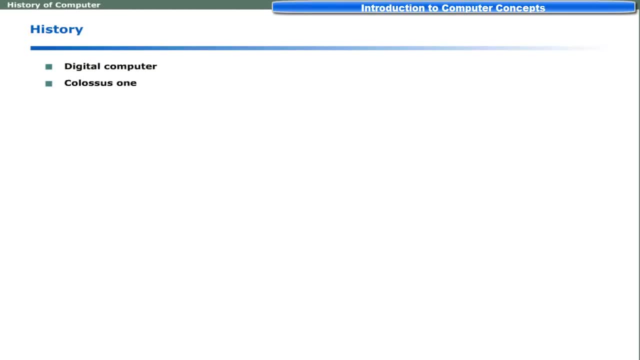 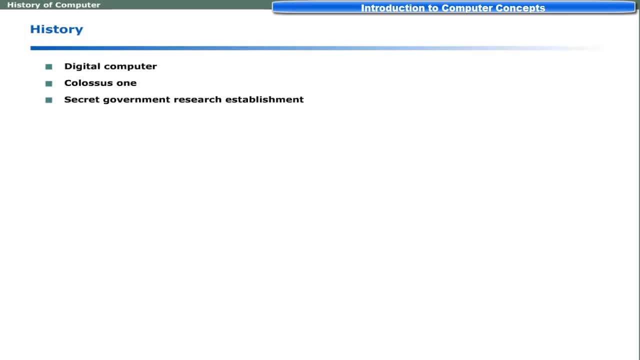 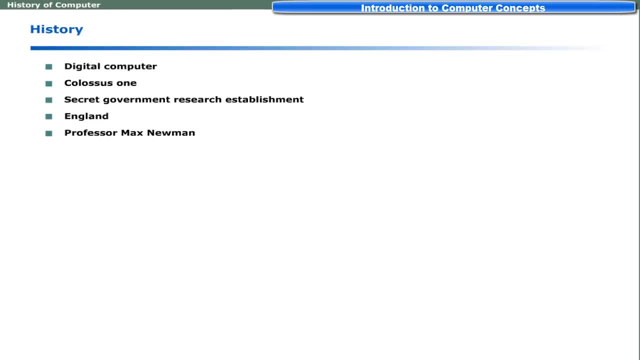 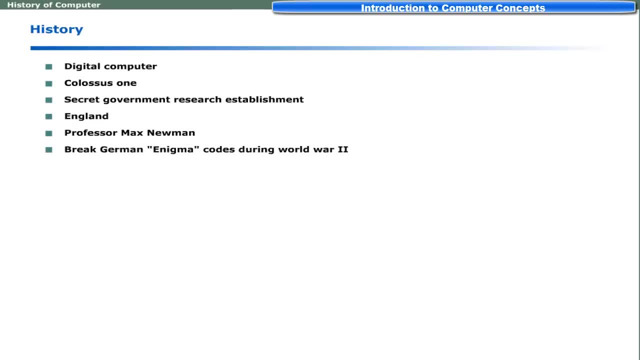 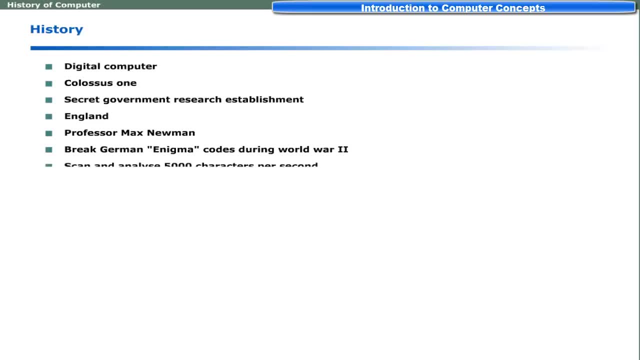 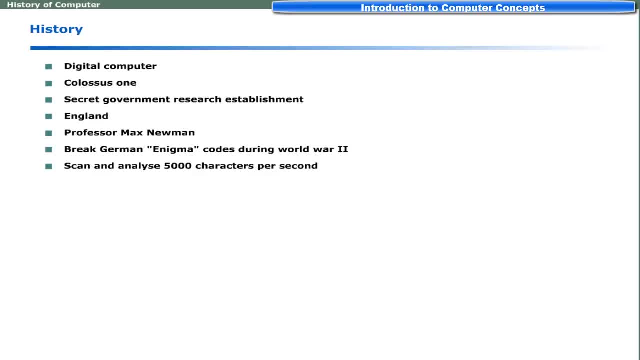 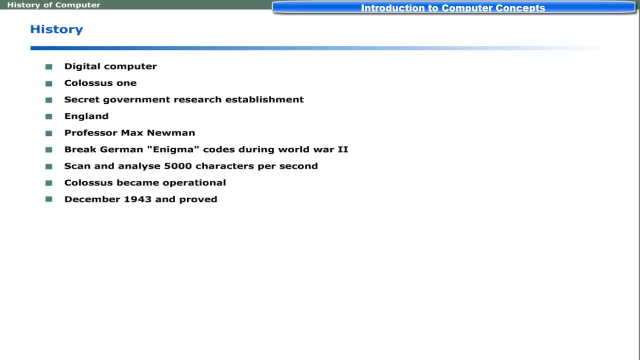 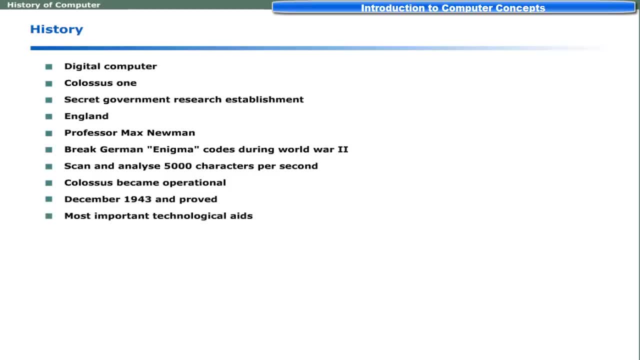 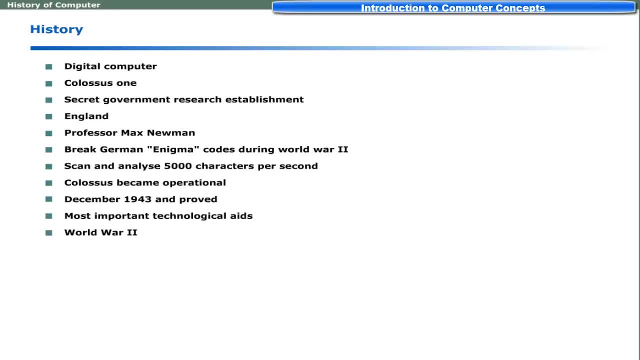 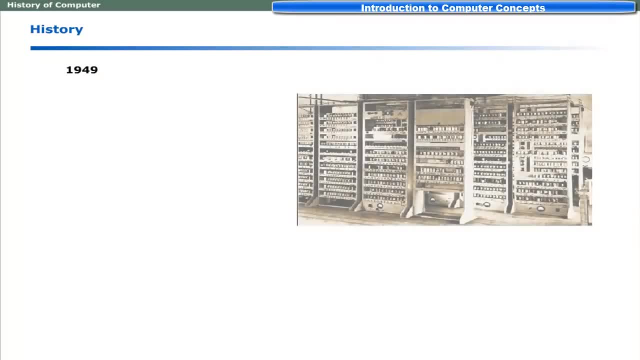 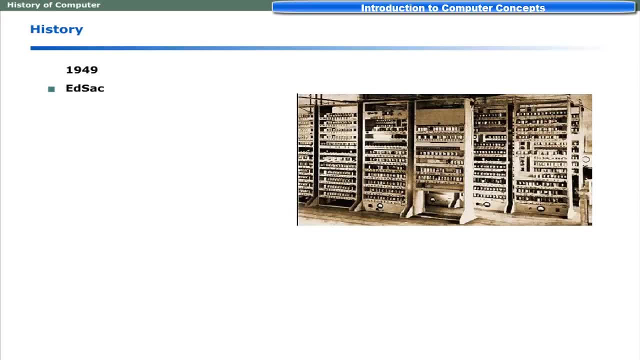 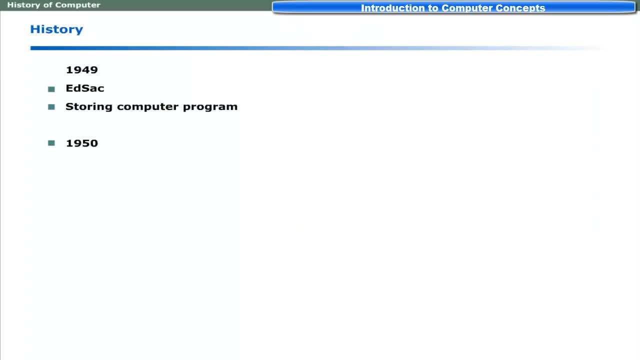 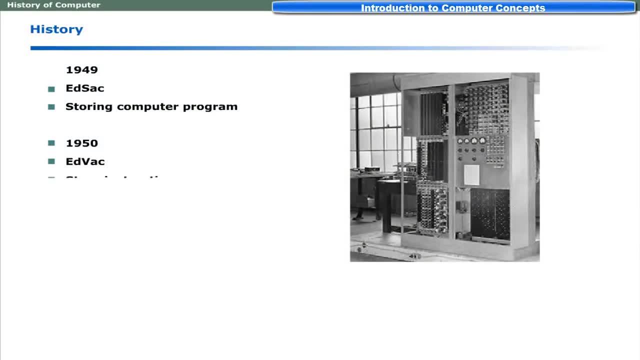 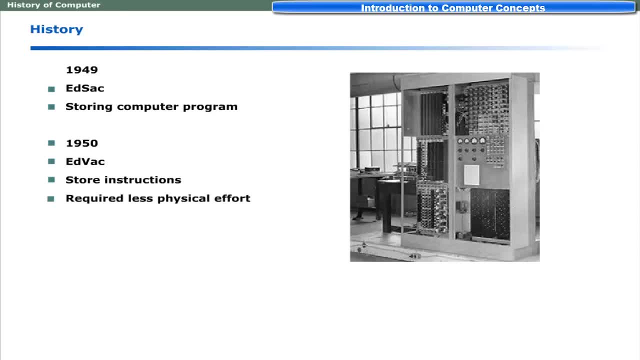 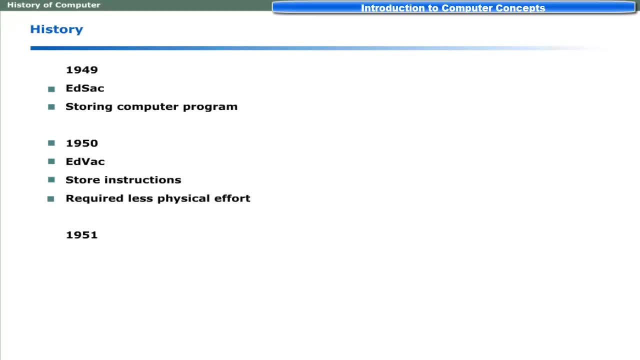 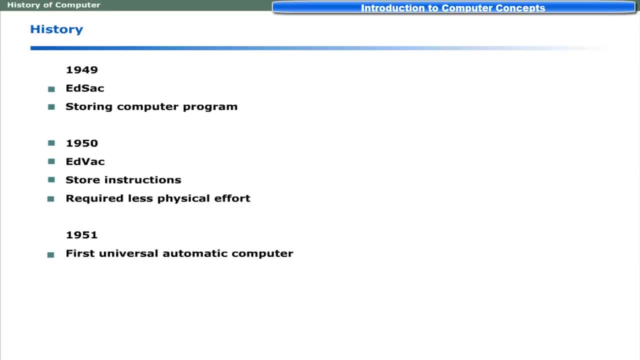 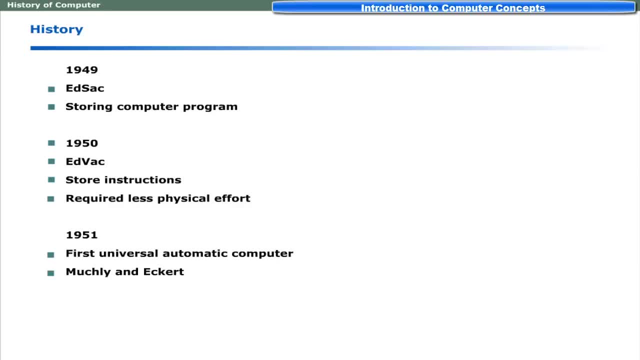 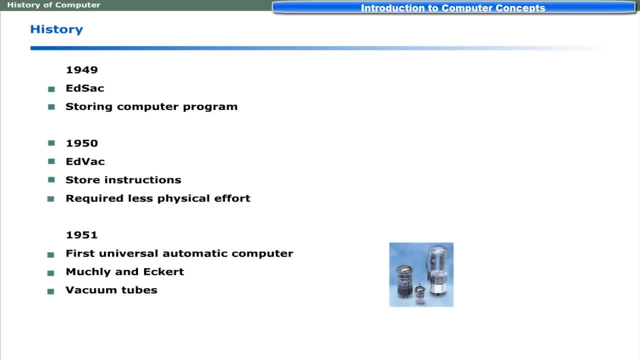 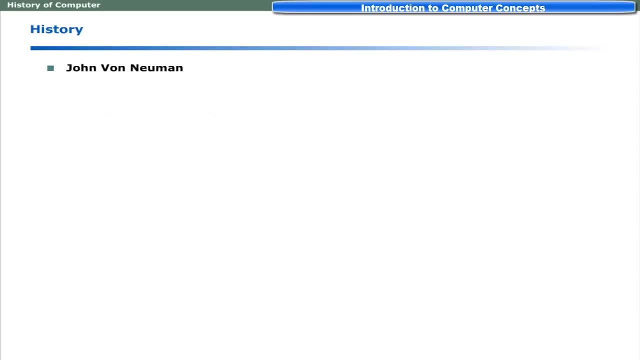 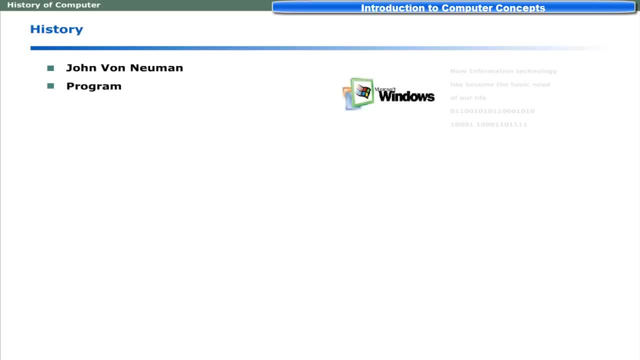 this was developed by John Murchley and John Presper Eckert. This was developed by John Murchley and John Presper Eckert. This was dost известing. Gideon and Saint James, The books of the three up there. 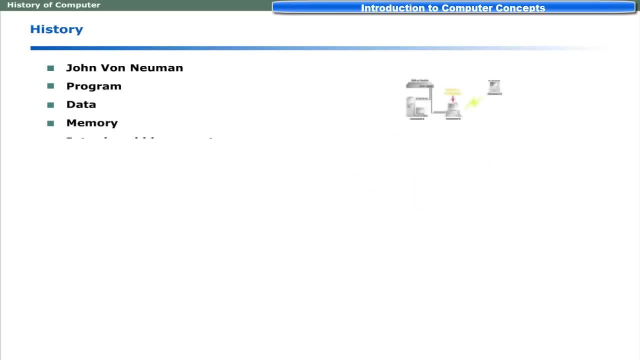 Excerpt from the book of Gideon, of the sequence: Why is it important for a book to form fortitude? What is it for? It's not all for, about fictitious. When the reader protects the readers about it, He is blessed. 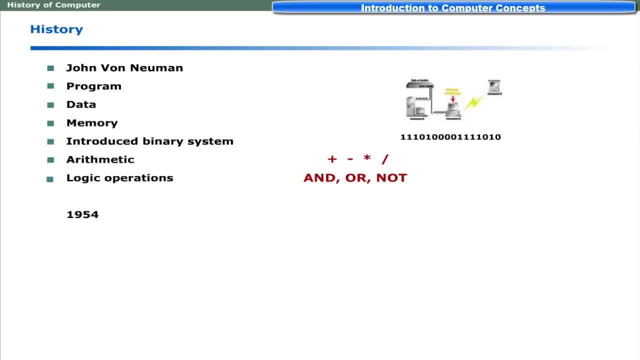 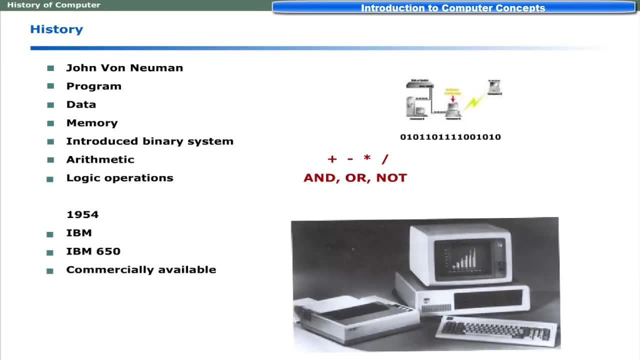 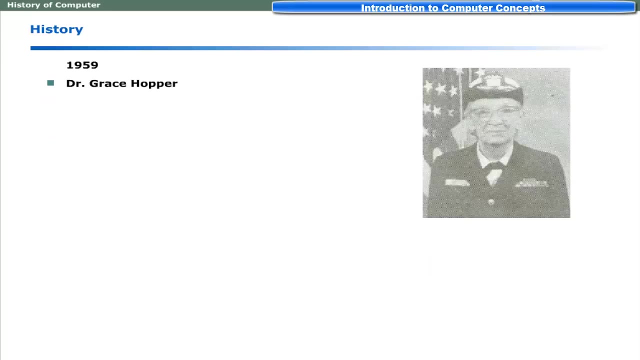 In this way, the reader place his full attention- And he is blessed- Here Jesus rose and he died. In other words, in another way, He is blessed and He was rewarded. Dr Robert Hopper conceived the idea of COBOL programming language. 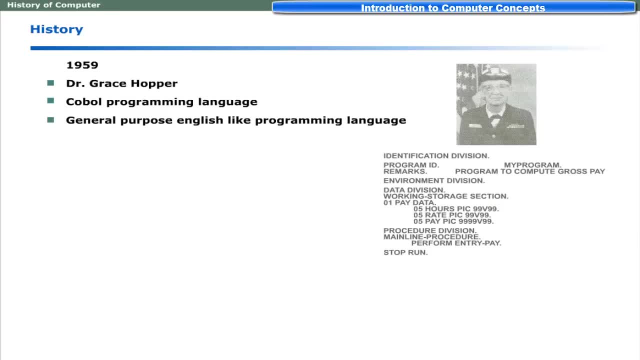 It was a general-purpose English-like programming language that is still used by many organizations. Dr Grace developed a compiler that translated programs written in COBOL to run on a variety of computers. She is also the pioneer to find first real bug in a computer. 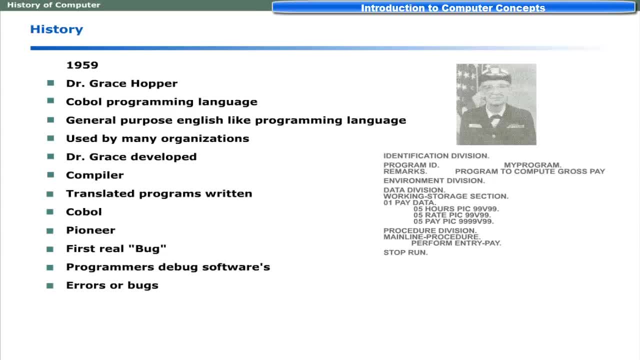 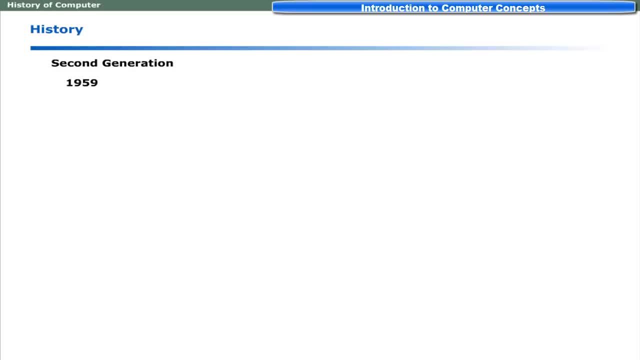 Programmers debug softwares to find out errors or bugs in their programs. Second-generation computers were introduced during 1959. These were built by using transistors instead of vacuum tubes. These computers were more powerful, reliable, less expensive and smaller in size than their 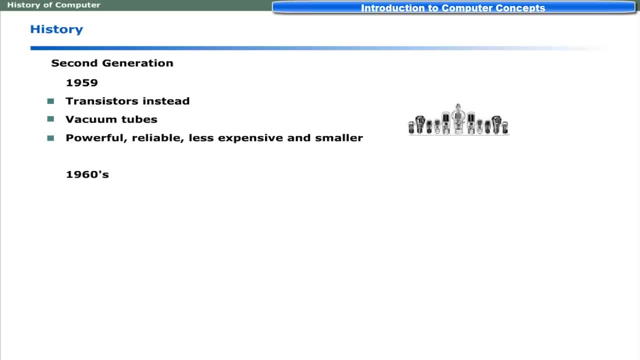 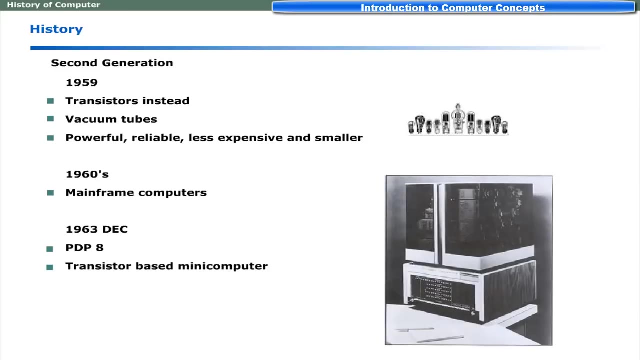 predecessors. Until early 60s, only large companies were producing mainframe computers. In 1963, DEC introduced PDP-8.. It was a transistor-based mini-computer. The demand for small computers tremendously increased for business and scientific applications. 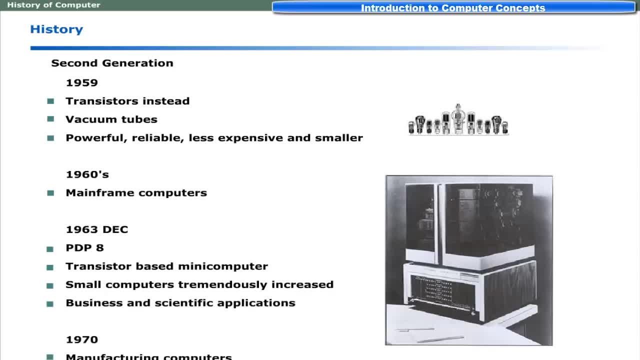 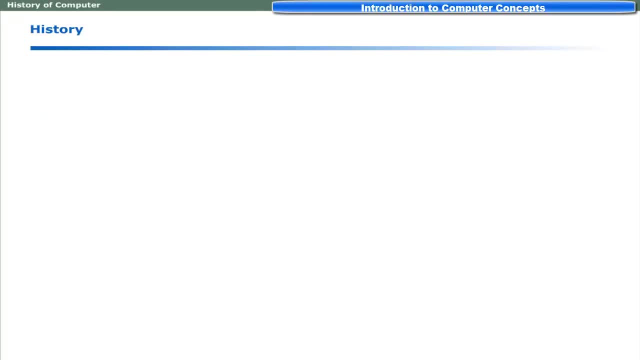 And by 1970, a number of firms were manufacturing computers, Dear learners. technology was rapidly changing and third-generation computers were introduced during 1964. These computers used large computers. These computers used large computers. These computers used large computers. Large computers used large-scale integrated circuits. 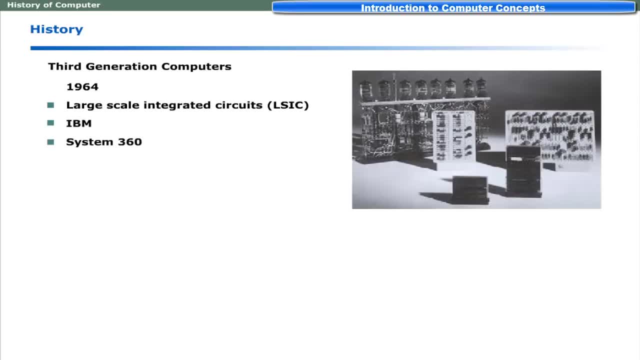 These computers used large-scale integrated circuits. IBM developed system 360 with the idea of upward compatibility that allowed companies to upgrade their computer systems without converting their data. Besides developments in hardware technology, scientists were busy in developing the techniques to interact with the computer to perform a variety of tasks. 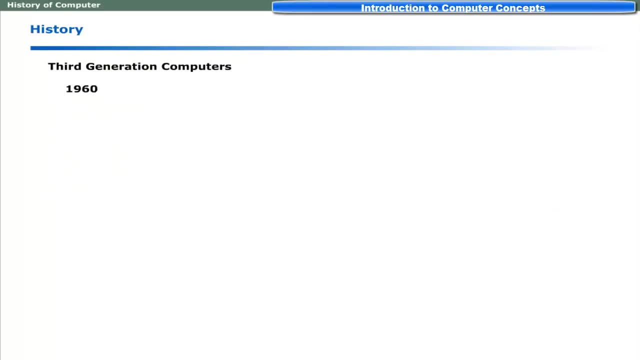 IBM developed a new system for standard computer technology, called computer and computer technology. as such, In 1960, Dr Thomas Kurtz and Dr Johan Kamini started developing a programming language and introduced BASIC programming language in 1964.. It became a popular programming language for business and scientific applications. 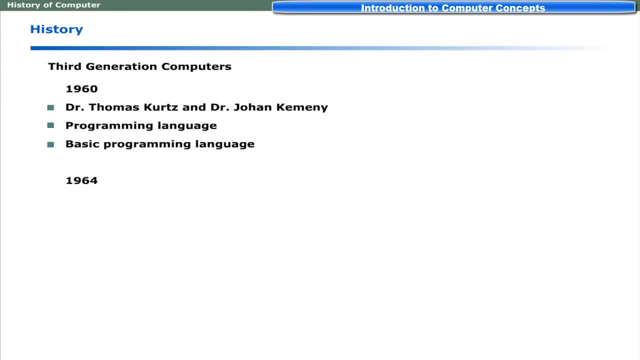 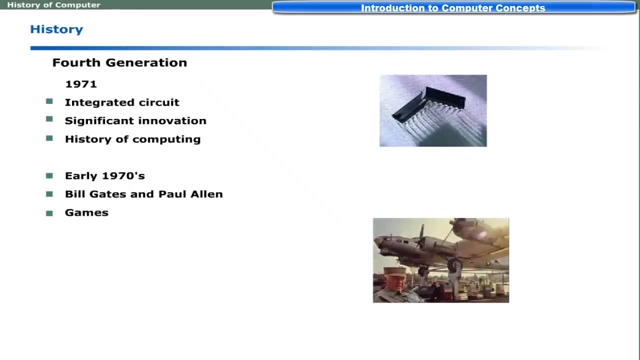 BASIC was supported on many types of computers. During 1971, fourth-generation computers were introduced with the introduction of integrated circuit. This was significant innovation in the history of computing. During early 70s, Bill Gates and Paul Allen were busy in developing games for personal computers. 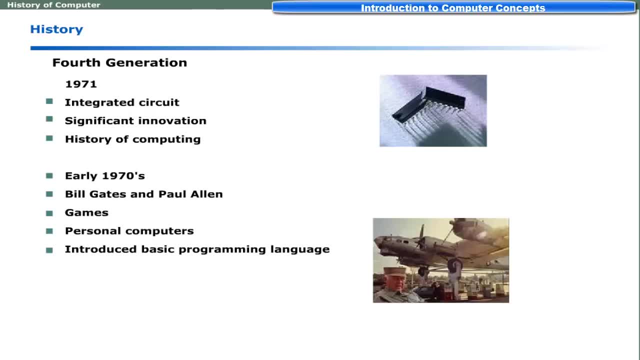 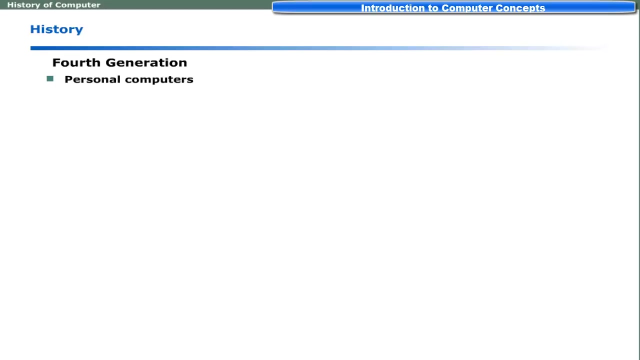 and introduced a BASIC programming language. They form today's most influential software. It revolutionized the idea of personal computing. with the introduction of Microsoft Disk Operating System, Dear learners, personal computers were not available. Apple II personal computer was introduced in 1975.. 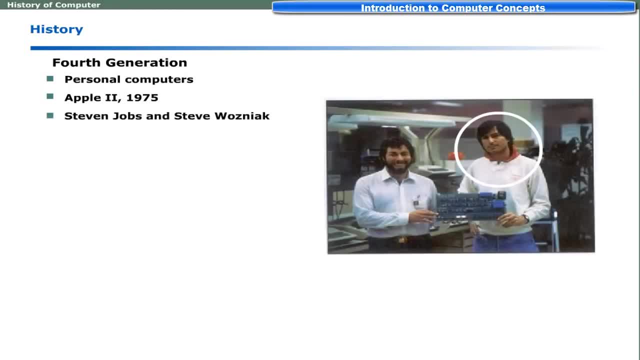 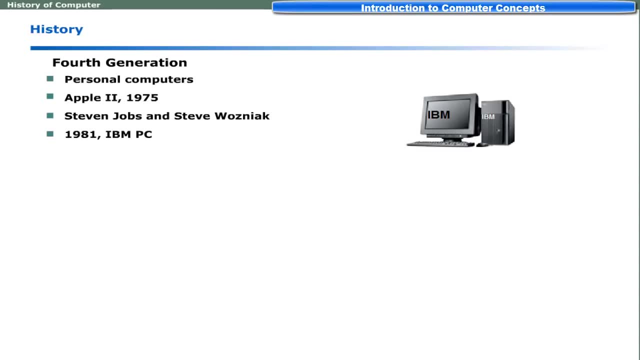 This was a prominent venture by Stephen Jobs and Steve Wozniak. In 1981,, IBM introduced IBM personal computer and many personal computers were sold by the end of 1982.. At that time, many other companies started manufacturing of IBM PC compatibles. 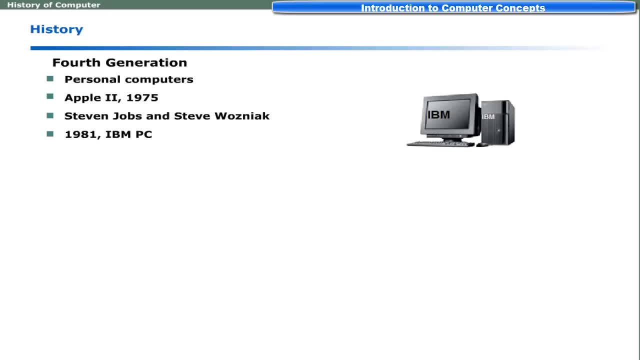 The use of personal computers had considerably increased in business, There was a tremendous need for business software. Mitchell Kappoor established Lotus Development company. Lotus Corporation introduced electronic spreadsheet application that boosted the sales of IBM PC and Lotus 1-2-3.. 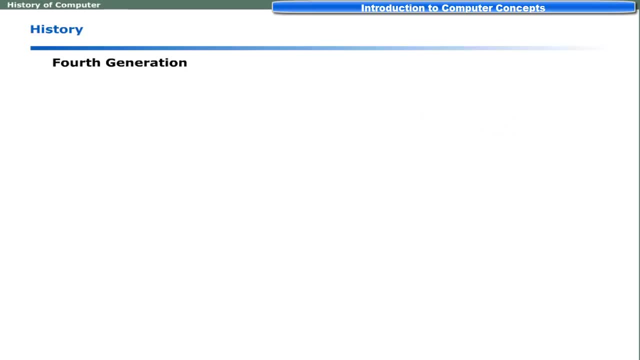 Dear learners, the credit for today's friendly, easy-to-use point-and-click graphical user interface goes to Apple Computer. Google's own computer is an important one. Google's own computer is an important one. GUI changed the human-computer interaction from text-based exchange mode to friendly WIMP interface.